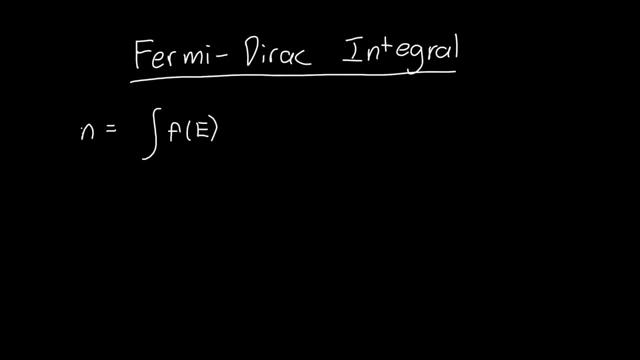 energies, the occupancy or the Fermi factor, the average number of electrons per state times the density of states G of E. And then we did this integral over energy And typically in introductory semiconductor physics you make the assumption: so this is EI, this is EC and this is EV. You typically make the assumption that the Fermi level 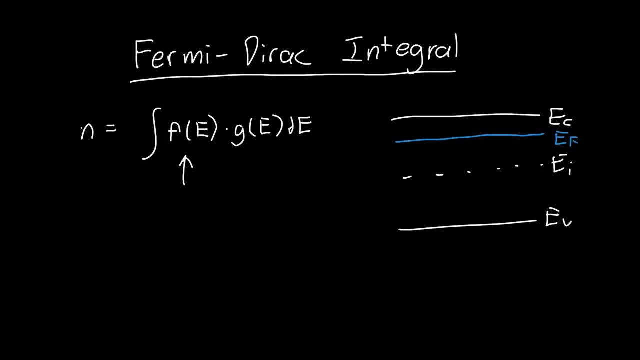 say- this is an N-type semiconductor- that the Fermi level distance from the conduction band is much, much greater, or at least greater than around 3 kT. So whatever the temperature is, it's going to be around 3 kT. So, whatever the temperature is, it's going to be around 3 kT. 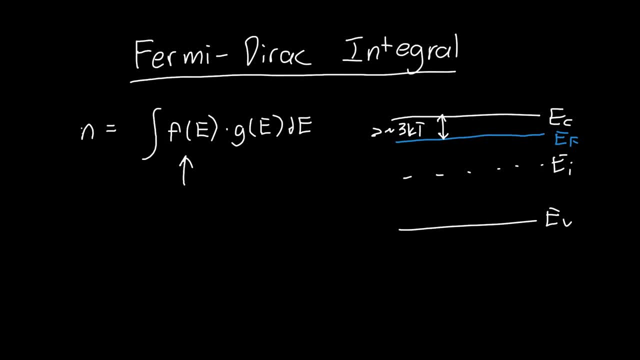 So, whatever the temperature is, it's going to be around 3 kT. So whatever the temperature is three times that thermal energy. And if you make that assumption, then this F of E simplifies into approximately a negative exponential, So it'll be E to the minus. 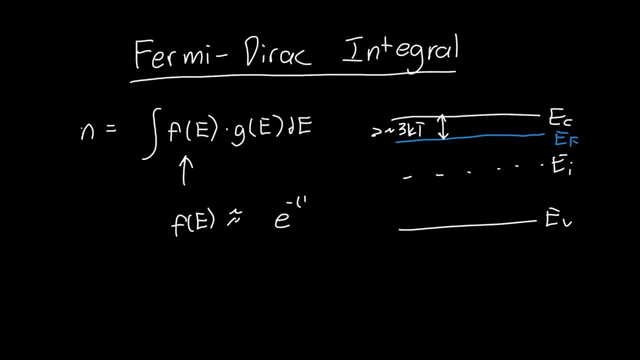 whatever energy you're integrating over, minus the Fermi energy over kT, And then that integral is tractable because, remember, our density of states is some prefactor that I don't remember off the top of my head: energy difference between the energy you're integrating over and the edge of the conduction. 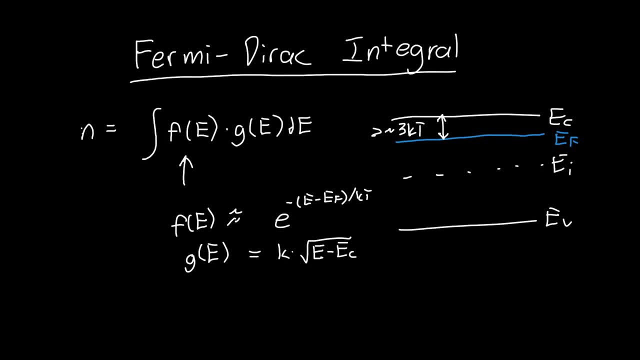 band And this integral is actually tractable if you're multiplying an exponential of energy by a square root of energy. But often this assumption is badly violated. So a lot of times in optoelectronics the Fermi level, or at least the quasi-Fermi level, is well above the conduction. 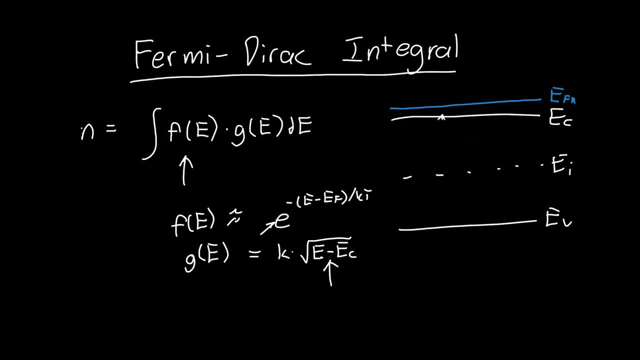 band. So clearly, this is a terrible, terrible approximation to make, And we need to actually evaluate this integral or find a better approximation for it, And so in this video, I'm going to be going through how we actually put this integral into a more tractable and 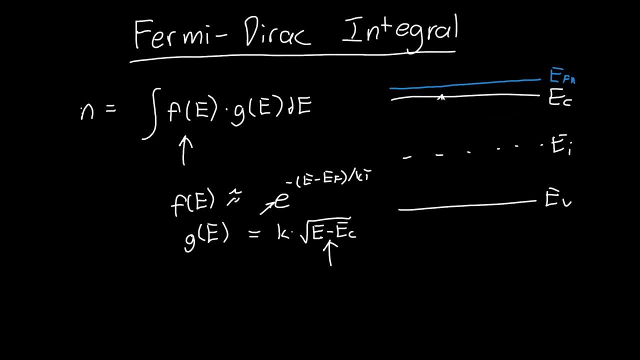 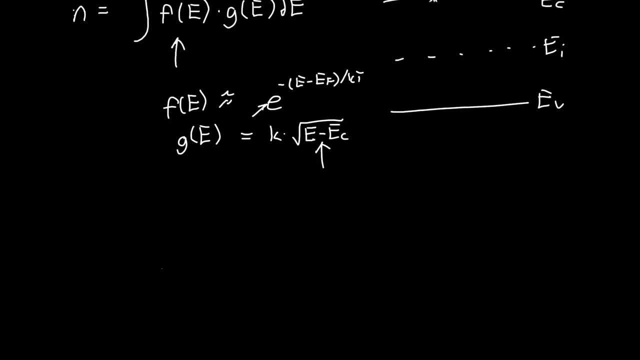 intuitive form and how we actually solve the Fermi-Dirac integral in practice. So let's just do, let's start with just a full frontal assault on the Fermi-Dirac integral. So let's just write out all the prefactors and everything. So if we do that, we get that n is. 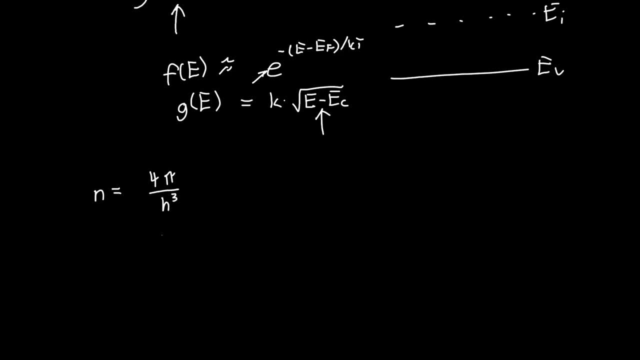 4 pi over h cubed times, 2 times the effective mass of electrons to the three halves. And then this is multiplied by the integral from the conduction band energy to infinity of. let's make the actual square root symbol of e minus ec. 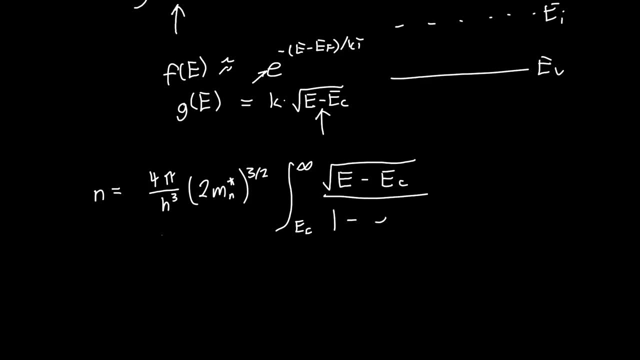 Over 1 minus e to the e minus ef over kt, And then this is integrated with respect to energy. Woo, That was a mouthful. And indeed this integral is gross, Like we've got so many things floating around. We've got the conduction band energy. we've got the Fermi energy, we've got 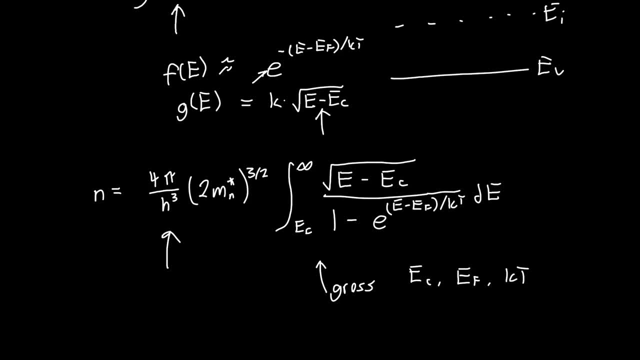 some kt's. we've got this disgusting prefactor out front that we're going to have to carry all over the place, And so we want to make this integral prettier. We want to make it more tractable, And the starting point for me is, when I look at this, I'm like: well, this integral inside has units of square. 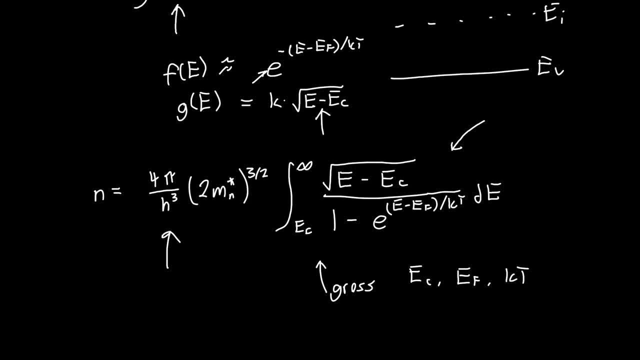 root of energy And once you do the integral, it'll have units of energy to the three halves, And that's just like no, that's disgusting. We would like to turn this integral into one that is unitless. So I'd like to turn this integral into one that's unitless And then out front. 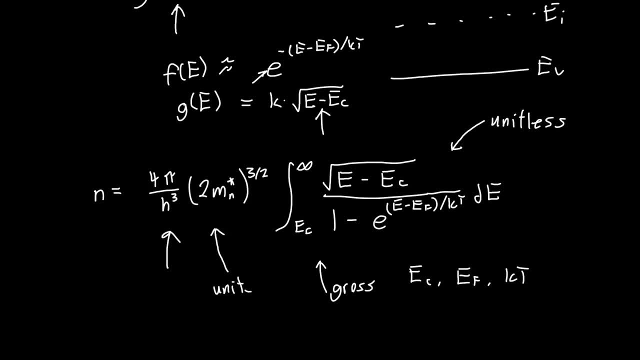 I can have some prefactor that has all my units And in this case it should be per centimeter cubed or in general per volume. So I would like the unit prefactor out front to mean something and the integral to just give me some unitless value, Because I like to think in terms of single. 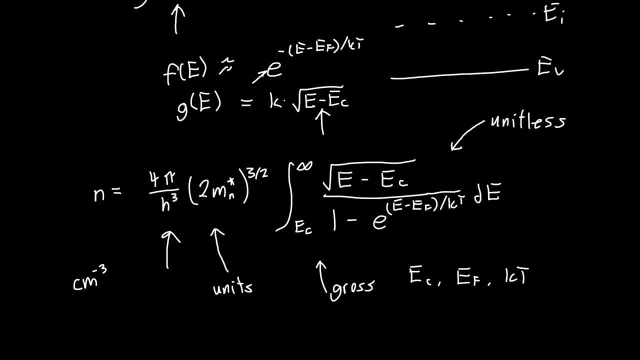 physically meaningful coefficients. So how do we make a substitution inside this integral to make the integral unitless? Well, we know that it's probably going to involve dividing an energy by kt, because that's how we're going to get rid of the units inside this exponential, Or that's how we're going to make 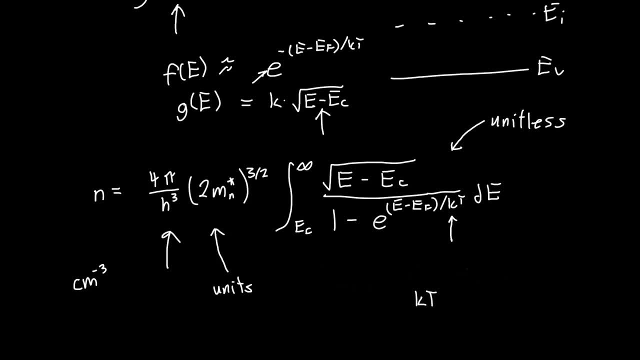 this exponential prettier And kt has units of energy, so that's convenient. We also want to get rid of this conduction band energy ec, because this whole integrating from ec to infinity- I'd really like this to be zero. If this could be zero, that would be great, And so I'm just going to make the substitution that 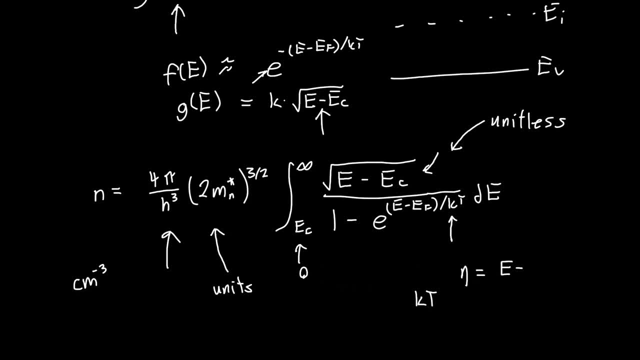 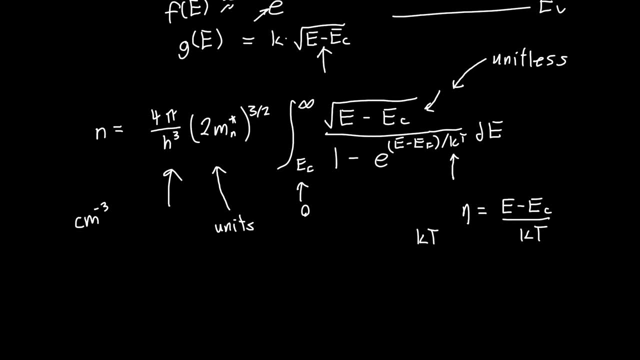 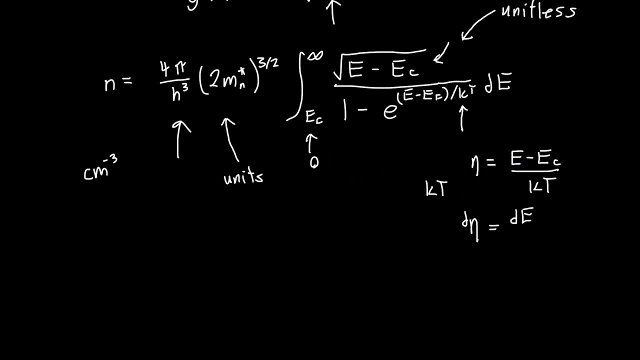 I'm going to call this variable eta. Eta is just equal to the energy that we're integrating over minus the conduction band, energy over kt. And if you make that substitution you'll see that d eta, or the differential with respect to eta, is just de over kt or solving for de. 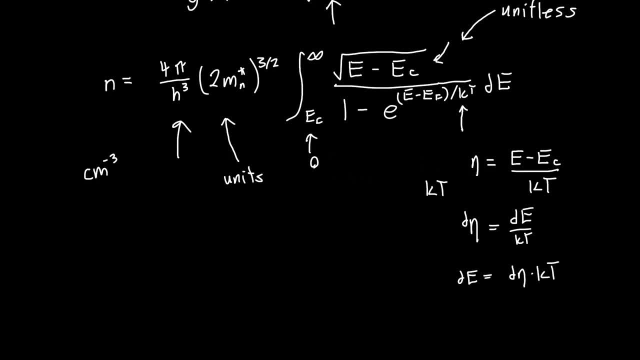 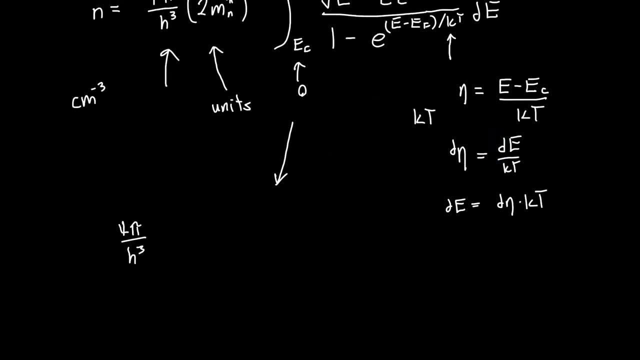 that's just equal to d eta times kt. So if we make the But, if we make that substitution and we rearrange the integral- I'm not going to go through the algebra here, but you can do it on your own- This prefactor out front will become 4 pi over h cubed. 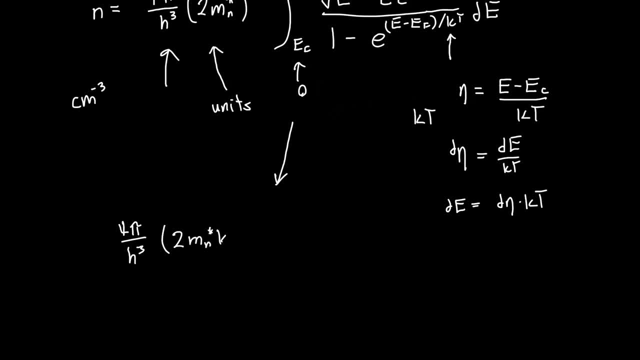 times, twice the effective mass times, kt to the three halves, And then this integral will now go from zero to infinity, which is really nice, And inside it's going to be the square root of eta d eta divided by 1, plus the exponential of eta minus. and this is where things get a little awkward. 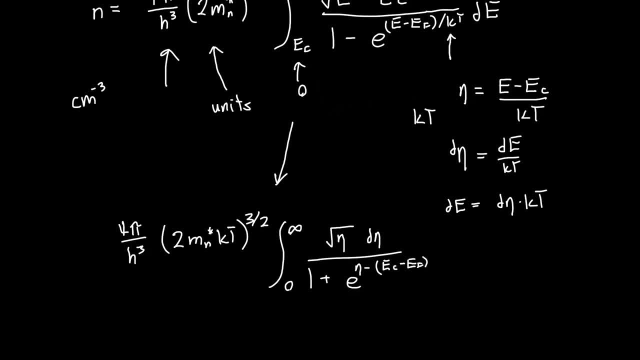 the conduction band minus the Fermi energy over kt. Now we can do a little better. We can just make this a little prettier by introducing some additional notation, because we see that this is a unitless quantity, this ec minus ef quantity, and it's just the difference between the conduction 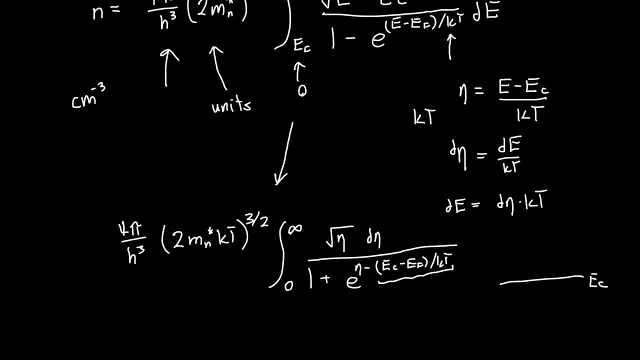 band level and the Fermi level. In this case this quantity would be positive if the Fermi level were above the conduction band level, which is unusual for traditional semiconductors but very typical in optoelectronics. So we're going to call this whole quantity eta f or, depending on who you ask. 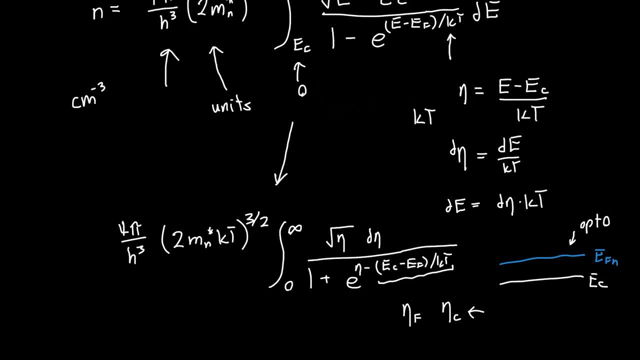 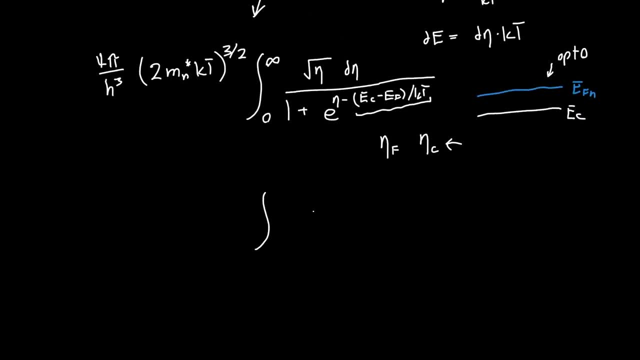 eta, c, c being for the conduction band. And so we can rewrite the inside integral. We can rewrite this inner term as just the square root of eta over 1 plus e to the eta minus eta, f, d, eta, And that's from zero to infinity. And then we've got this pre-factor out front. So what do we do with? 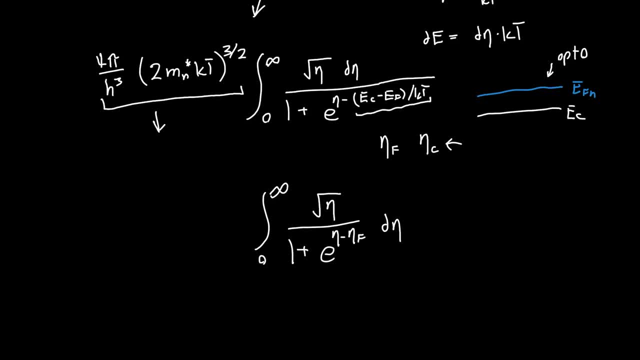 this pre-factor. Well, since the integral is unitless, this pre-factor has units of per volume or per centimeter cubed, And so you might just be tempted to call this some n-effective, so some electron density, because it's got the same units as electron density. It turns out this is actually 2 over the. 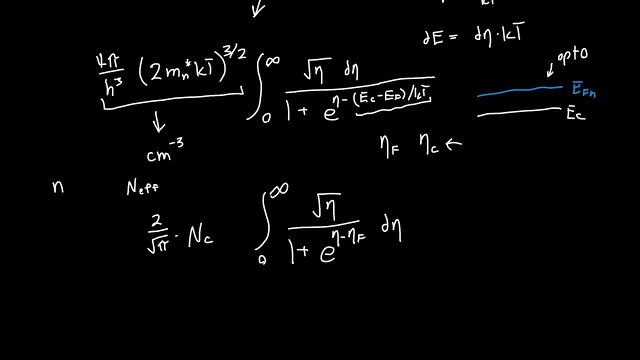 square root of pi times nc. where nc- and let me move this over so it's actually next to the integral nc- was our effective density of states. So 2 over root pi times nc. And if you haven't seen nc before, 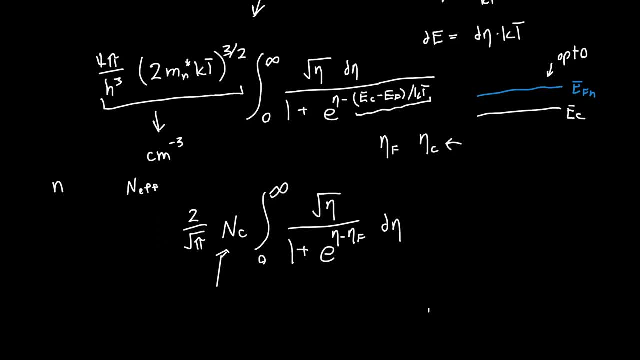 this is a parameter that's defined in Nieman as well as a bunch of other things. So this is a parameter that's defined in Prine, like many other semiconductor physics textbooks, which is used to sort of encapsulate all these nasty coefficients, So Planck's constant Kt, the effective mass, And so it's very common and 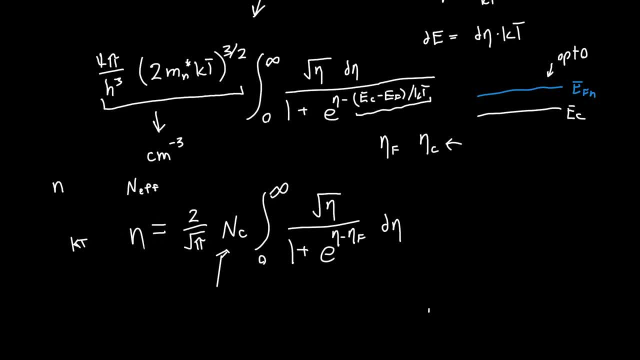 shows up quite a bit, And so this is our electron concentration n. This is the nicest form I've been able to find this integral when you have to deal with the integral directly. But you might say: well, now I have this. 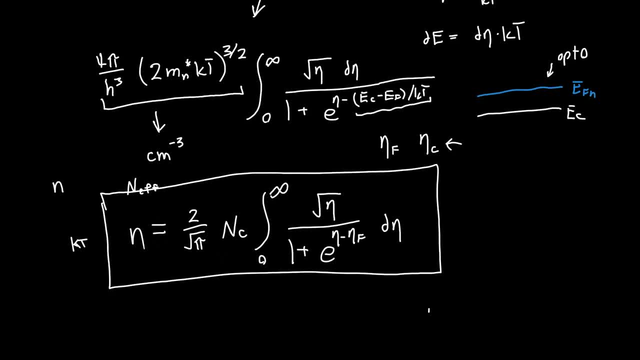 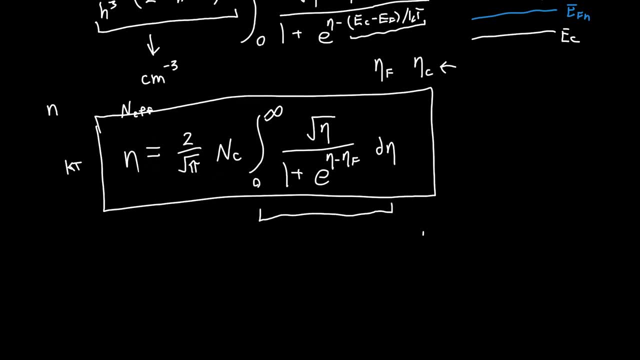 integral. Well, what is this integral? While I'm just taking a little break here, I Jordan great like you've still left us with an indefinite integral, But this term right here. this integral is, first of all, it's only a function of one variable. 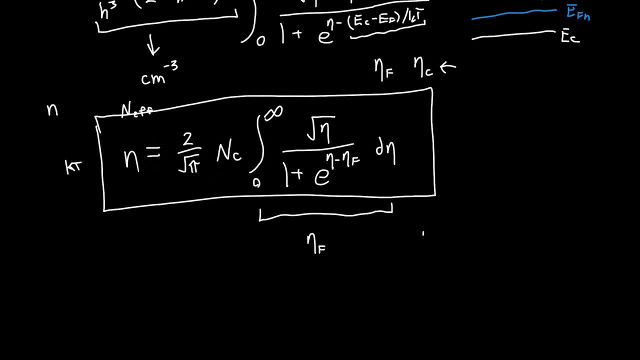 So it's only a function of eta F or eta C how far away the conduction band edge is from the Fermi level or the quasi Fermi level for electrons, And so that's really nice, And so we often write this as two over root pi. 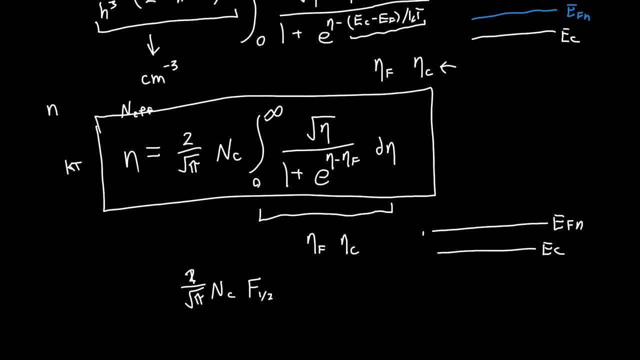 and C times this F one half function, which is a function of eta F And F one half is the Fermi Dirac integral of order one half. So order one half And this integral is actually tabulated. So if you have Mathematica, for example, 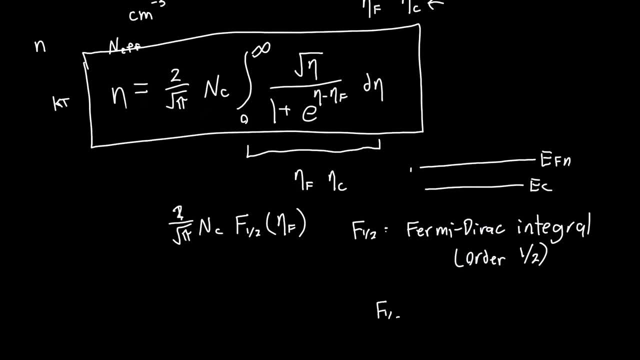 you can evaluate F one half. You can say what is F one half at a value of zero, or at a value of one, or at a value of two? Is this eta? F is a unitless quantity. remember, it's the distance between EFN and EC divided by KT. 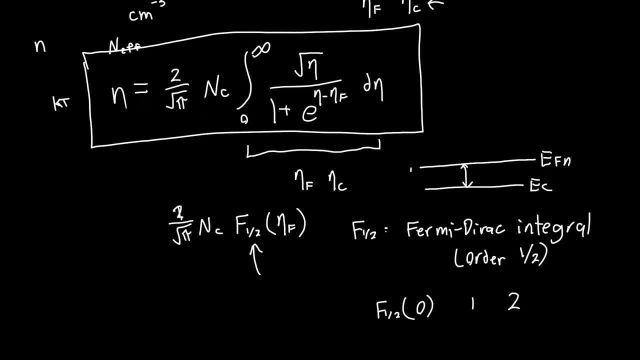 So this is just a known function like any other. I think MATLAB has it as well. You can just evaluate it at certain values: eta C or- uh sorry- NC. This is known. This is just a material property, So this depends on your material. 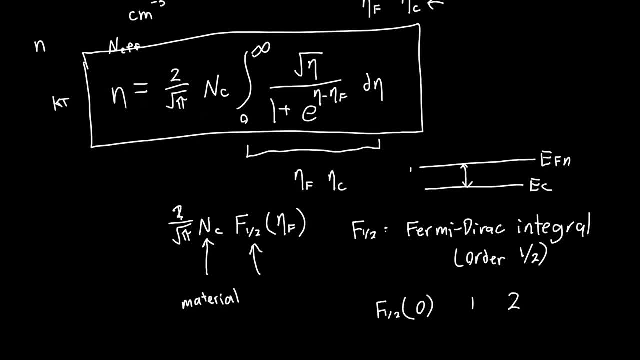 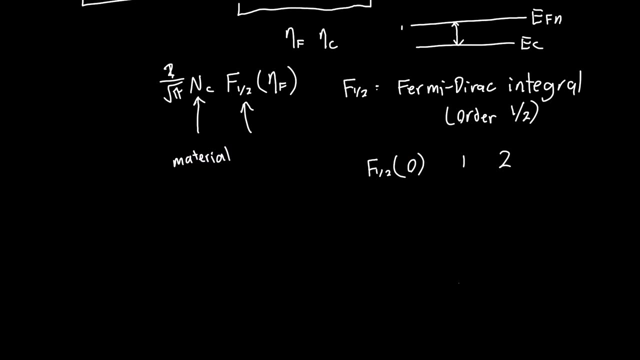 So, whether it's silicon, germanium, gallium, arsenide, this NC value is just tabulated, And so this is a very easy, very elegant way of expressing the carrier concentration. But the real power of this and one of the reasons it's really cool. 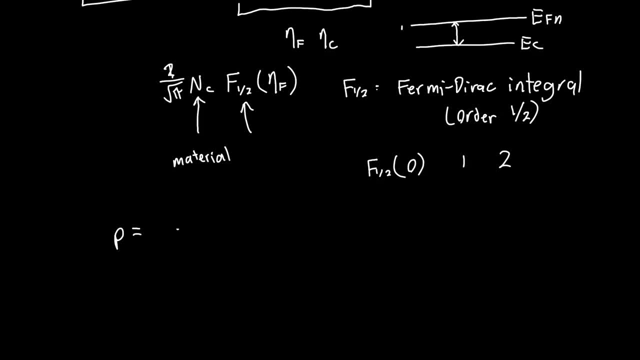 is because you can do the same analysis and you'll get that the whole concentration is equal to the same Thing, with a couple of caveats. So instead of NC it's NV, And instead of this eta C term. so it's not C anymore. 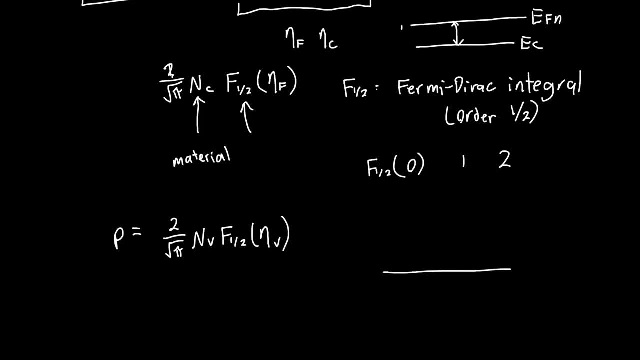 this is eta V. So eta V is just the distance between the bottom of the valence band EV and the Fermi level EFP or the quasi Fermi level EFP. So if we draw out the full bad diagram, we've got EC, we've got our intrinsic Fermi energy. 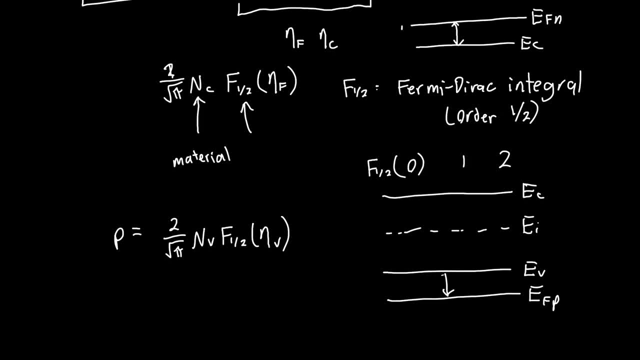 This assumes so eta V is positive when EFP is below EV, And so this gives you the whole concentration, This gives you the electron concentration, And they can just be evaluated. They can be solved numerically, but there's also approximations. 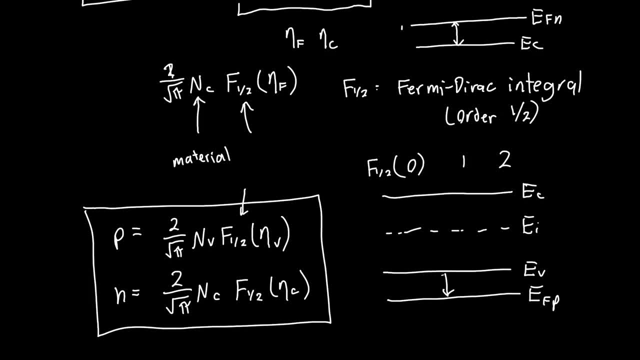 for these Fermi Dirac integrals. So this F one half term. So, for example, when this distance is much greater than 3KT, there's also an approximation for this Fermi Dirac integral. So this F one half term. So, for example, when this distance is much greater than 3KT. 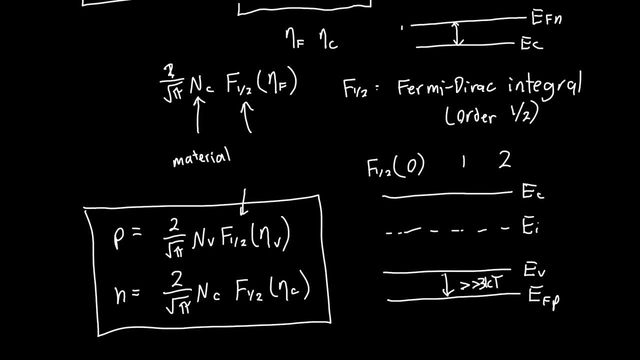 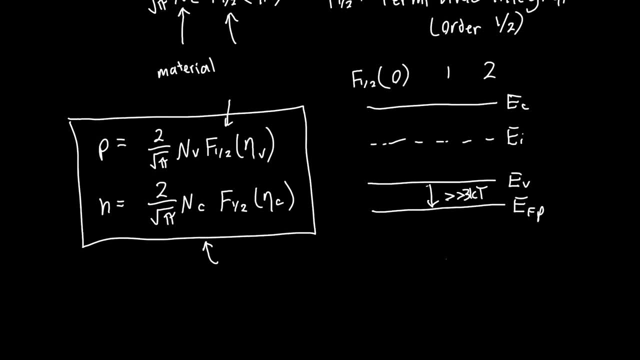 So, for example, when this distance is much greater than 3KT, then we can make a different approximation for the Fermi Dirac integral, And this form of calculating the electron and hole concentrations is also really useful in 2D, 1D and zero dimensional systems.